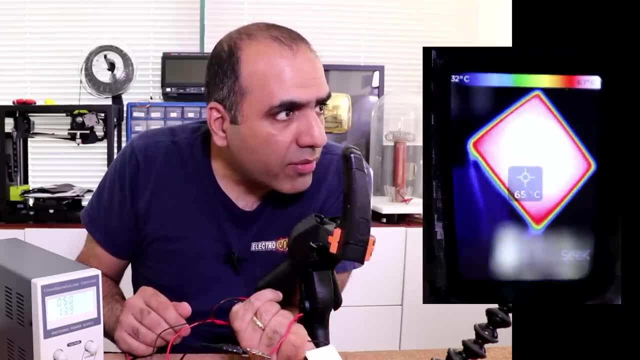 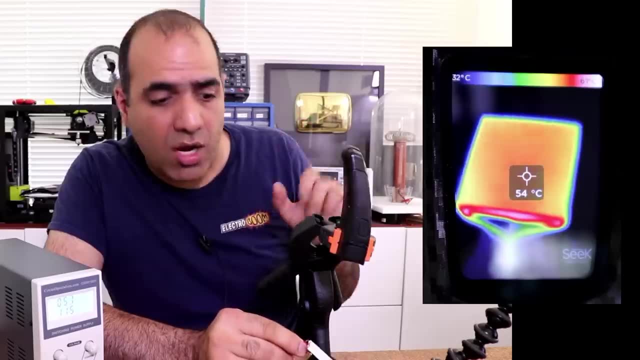 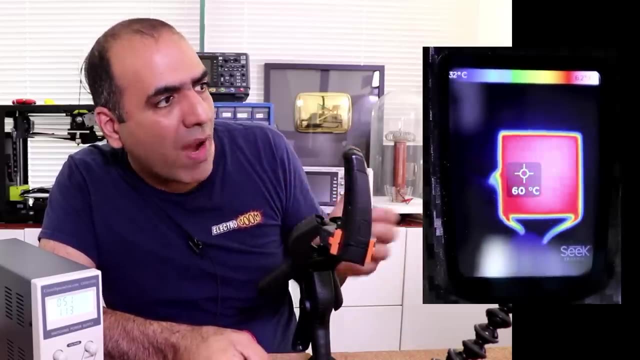 cooling down and that side is heating up. if I let it run for a while, the cold side heats up too. but it seems like the device is keeping the temperature difference constant around 30 degrees at 5 volts, and the temperature difference between the two surfaces is power dependent. so at maximum power the 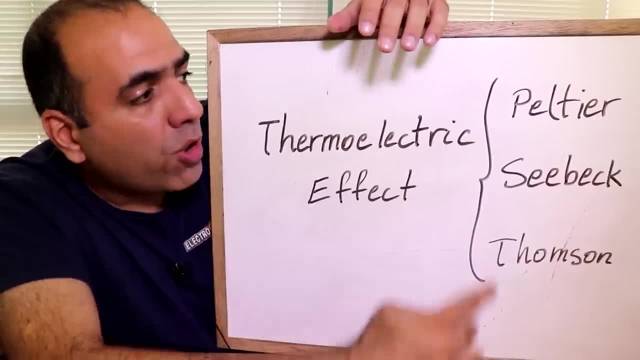 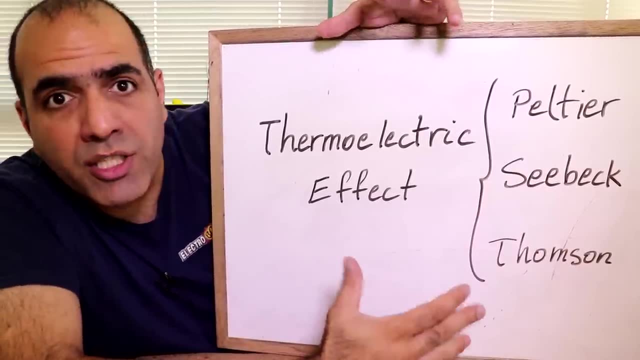 difference can be 60 to 70 degrees. these things work based on Peltier effect, Seebeck effect and Thomson effect, which is basically the extension of Seebeck and Peltier effects, and all these are different manifestations of the one thing, that is, the thermoelectric effect which happens when two conductors with 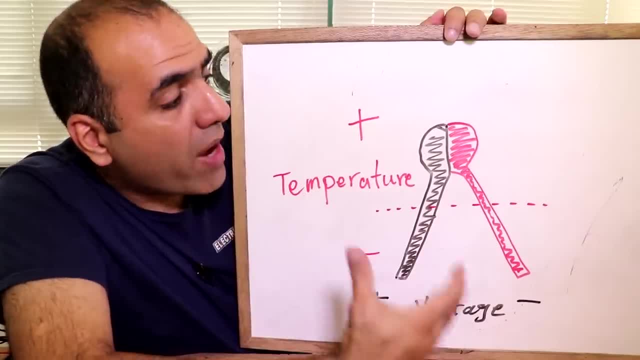 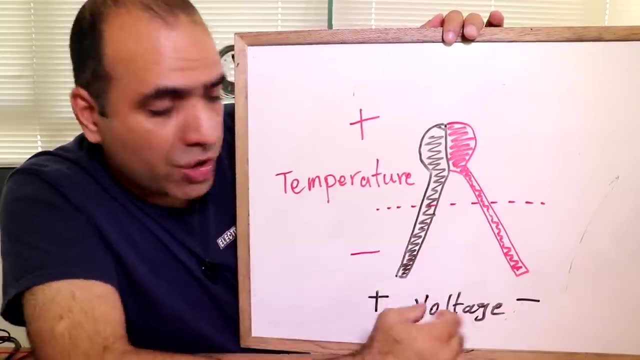 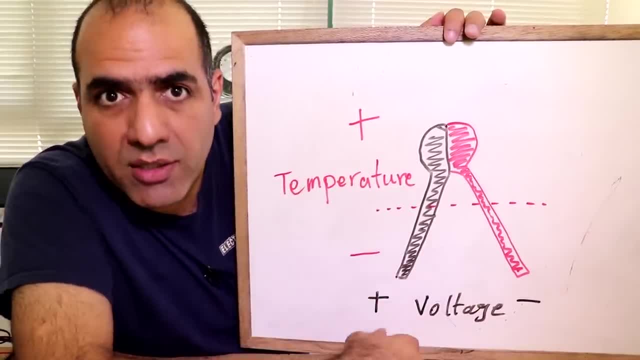 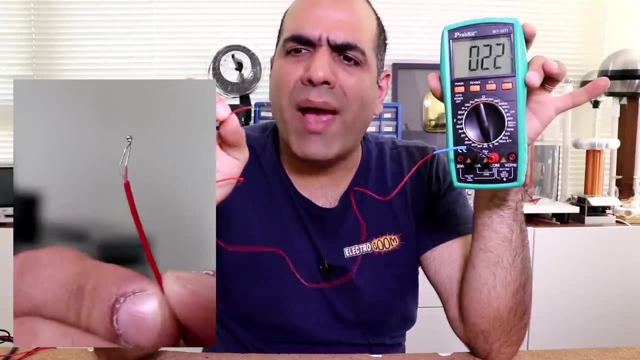 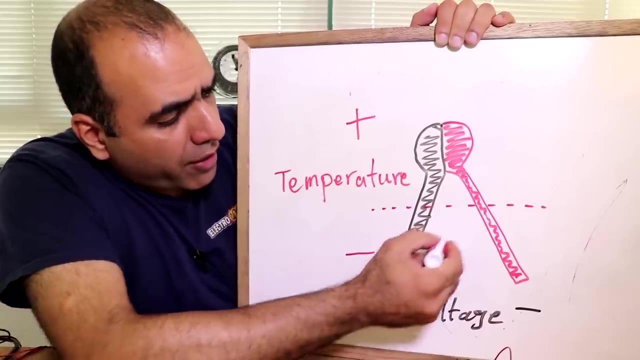 And there's a temperature difference between the junction of two materials and rest of it, a voltage is created across the junction and acts like a generator. the voltage is typically very small, in order of micro volts, and increases with more temperature difference. measuring that tiny voltage, you can measure the temperature. that's what they do in thermal couples joining. 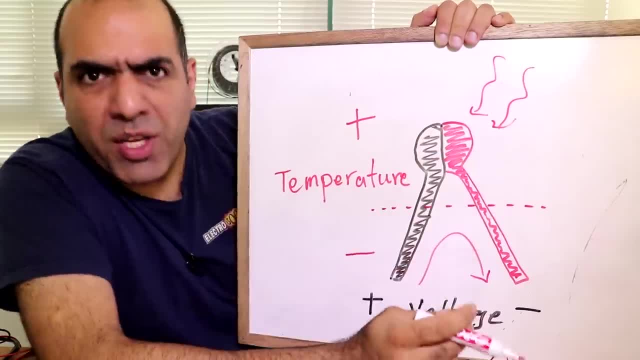 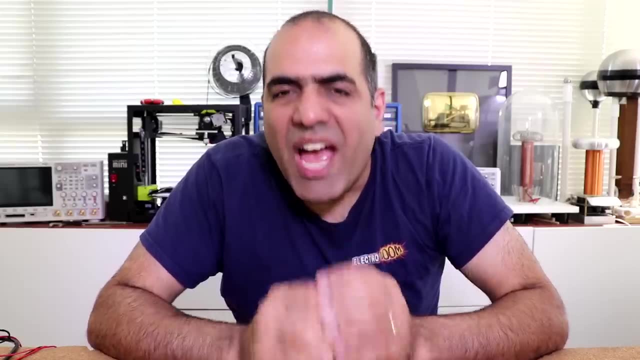 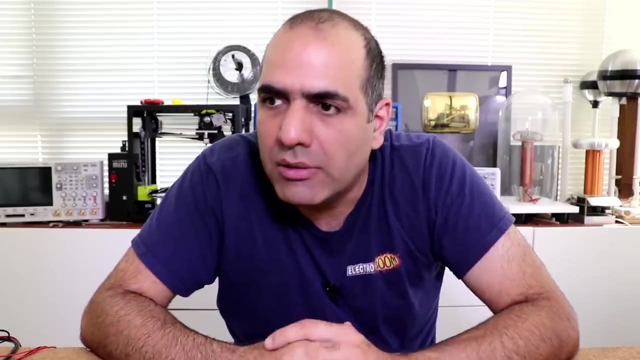 joint. it can cool down and absorb heat, or it can heat up and radiate heat, depending on the direction of the current. The problem is that I have no idea what happens in atomic quantum level, that passing electricity through two material can cool it down. I read somewhere that the electrons move the 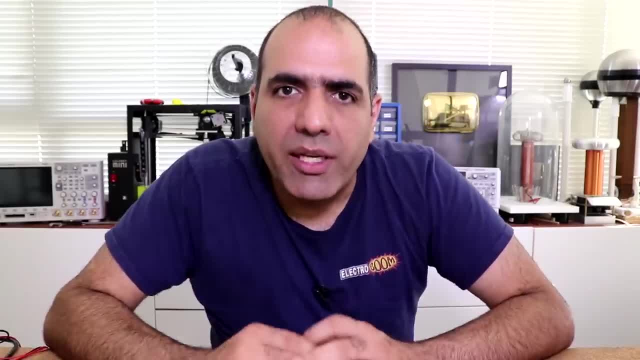 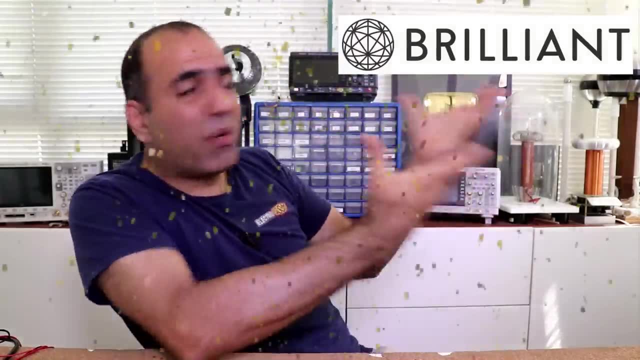 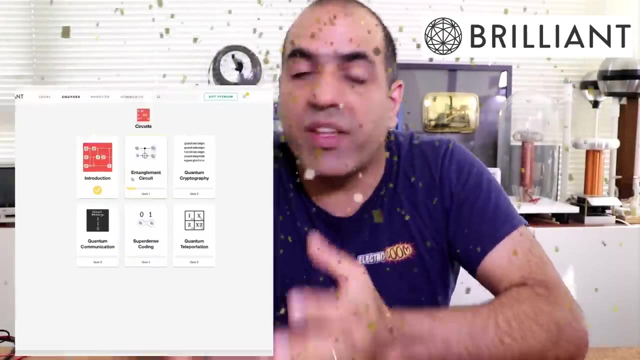 heat away. What the hell does that mean? If you know a good explanation, please leave it in the comments so I learn it too. Or if you want to learn math and science, then check the sponsor of this video, brilliantorg. Such professional, much interactive, tons of math and science courses with interactive problem. 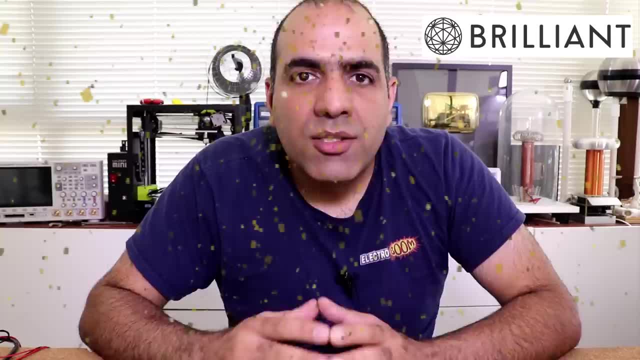 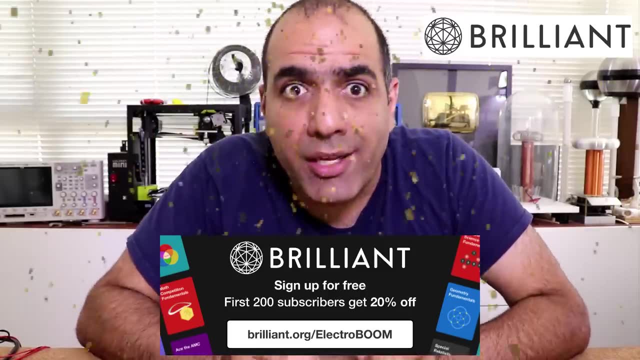 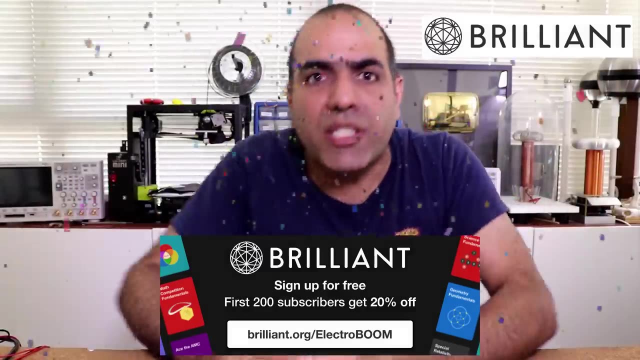 solving and quizzes to make sure you learn what you want better. So sign up for free at brilliantorg slash electro boom to get access to a lot of free courses already, But using my link, you get 20% off of the annual premium subscription. that gives you full website access for less than $10 a month. So 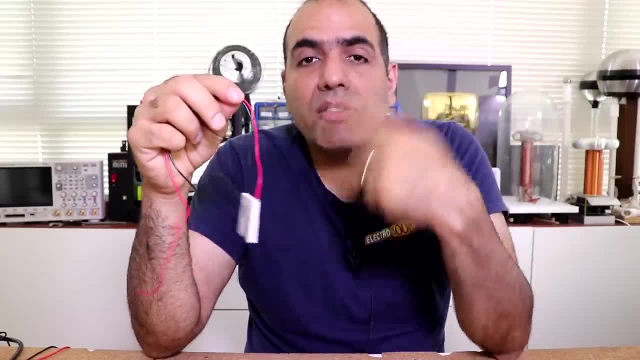 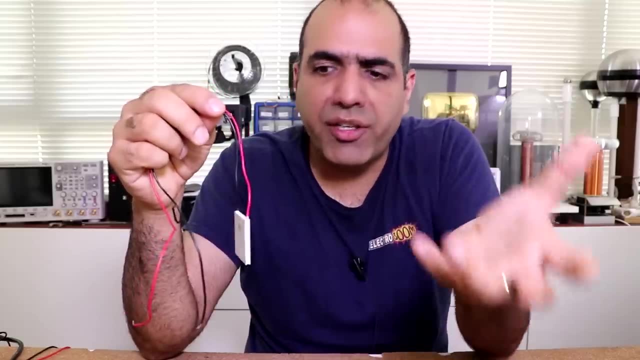 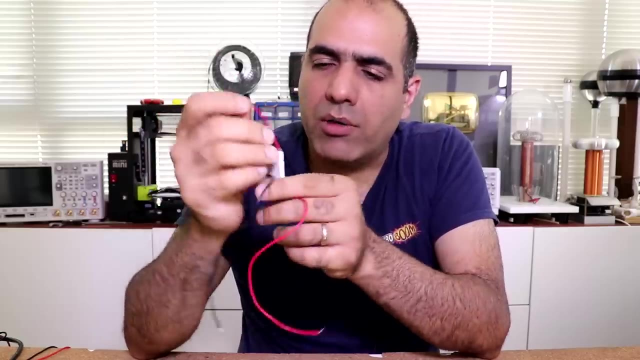 let's get started. This device is fascinating For whatever reason. when you run current through it, it pushes heat from one side to the other, creating a temperature difference Like if both surfaces start at 30 degrees Celsius. running current can make one side zero and the other 60 degrees, But it also wastes tons of power: 50 watts. 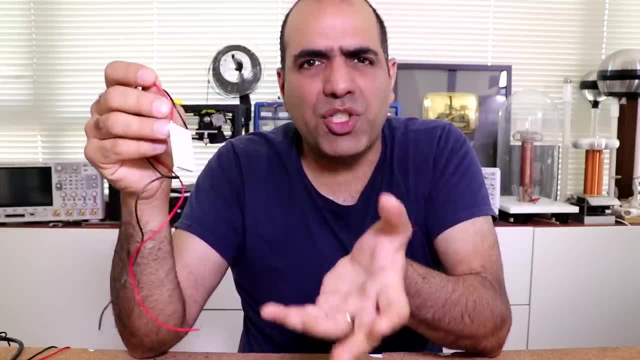 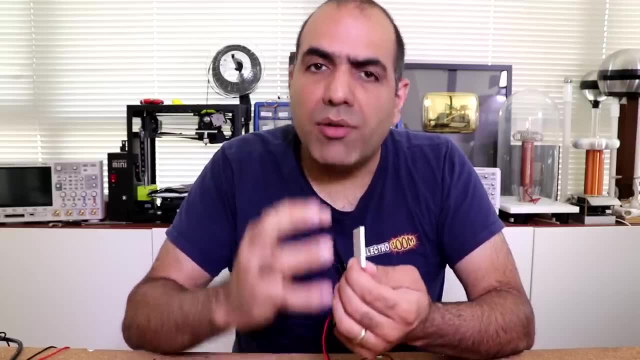 max for this guy. So it heats up quickly while the temperature difference remains around the same. So one side could be 100 degrees and the other side 40. But if I can somehow cool down the hot side to say 50,, that would be great. So let's get started. 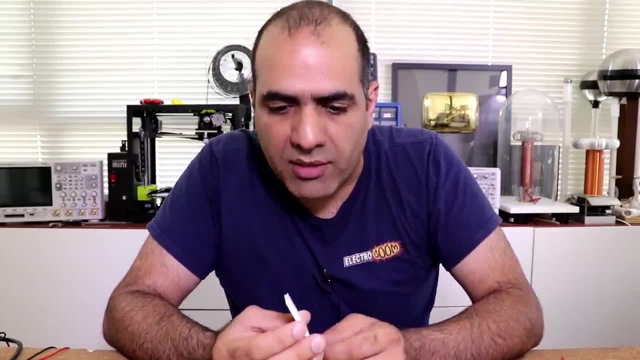 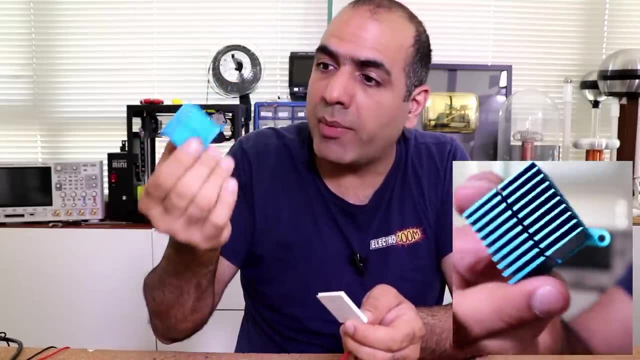 Okay, let's give it a try. So the cold side could be minus 10 degrees. The cold side would suck the heat from the environment and pump it to the hot side. That's why I bought a bunch of heat sinks to experiment with. So I attached the device and heat sink using a thermal. 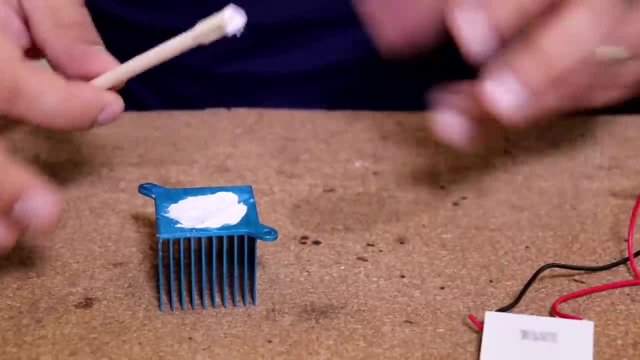 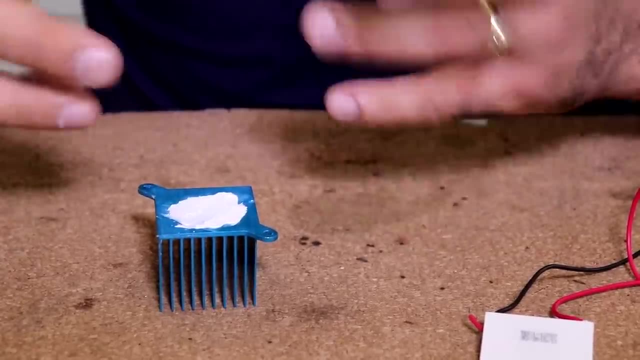 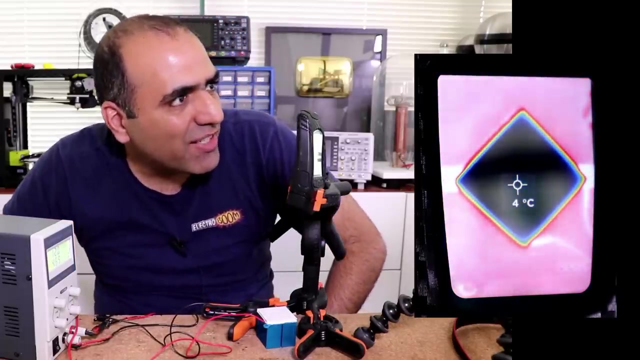 compound that fills the gap between the two and provides a very good thermal conductivity. The metal heat sink with so many fins creates a large surface area to transfer heat to air better and cool down. Okay, let's give it a try. Oh, look at that, The surface is getting colder, Great. But as the heat sink is getting 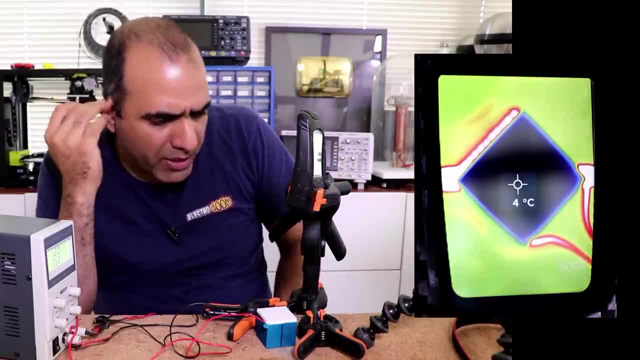 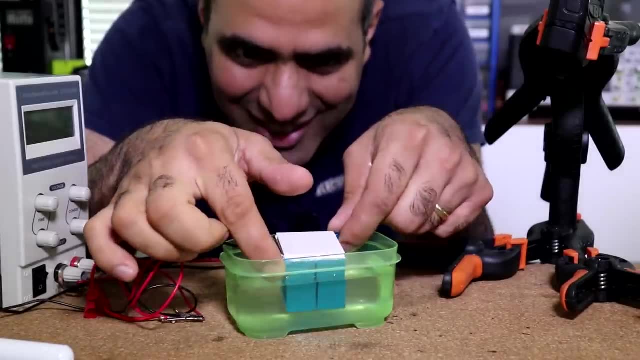 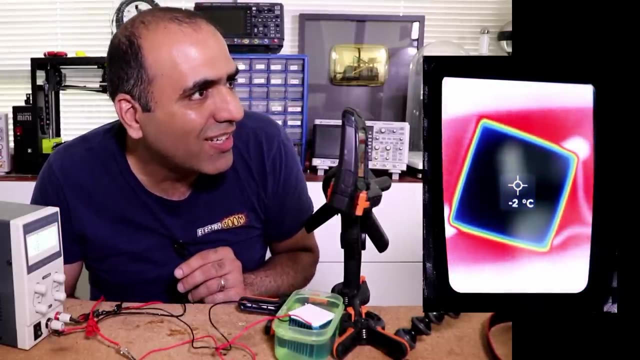 warmer. the cold surface is going up too, Which means we have to blow air with a fan on the heat sink to keep it cold. Or, even better, just place the heat sink in cold water And we power it up. And there it goes, Of course, as the water slowly heats up the temperature. 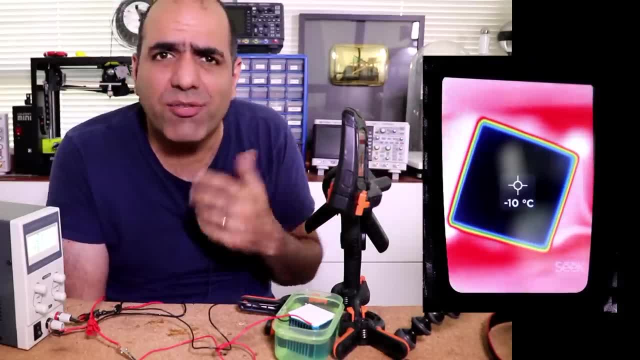 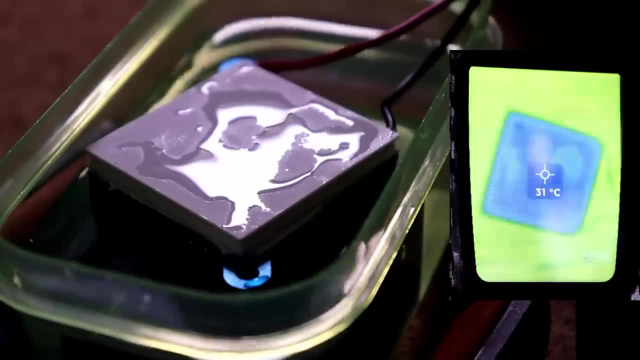 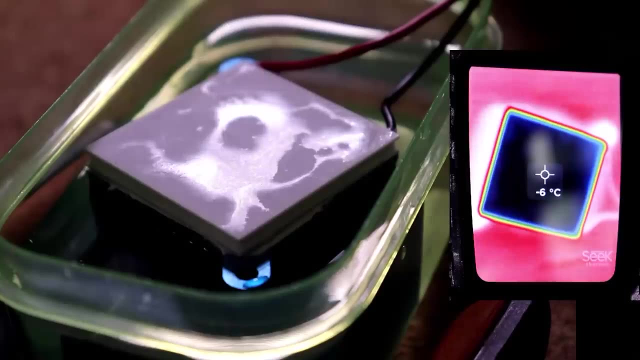 too. Running cold water would help, but that wastes a lot of water Minus 11 degrees. Let's add some water to the surface and power it up and see what happens And zip It all freezes. And if I disconnect the power, BAM It heats right. 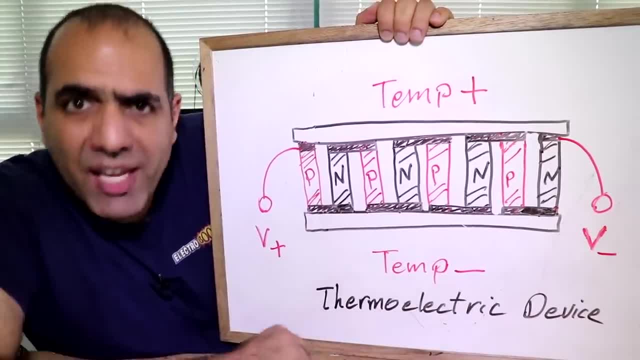 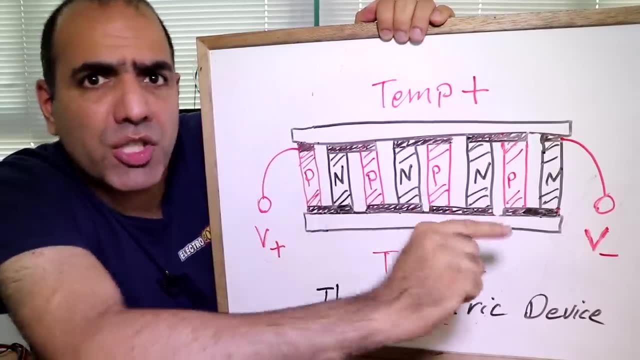 back up These peltier devices, or shall we call them thermoelectric devices, work on the same principles I talked about, But instead of one junction of two different material, there are many junctions placed in series like this between two surfaces made of P and N semiconductors Running current through 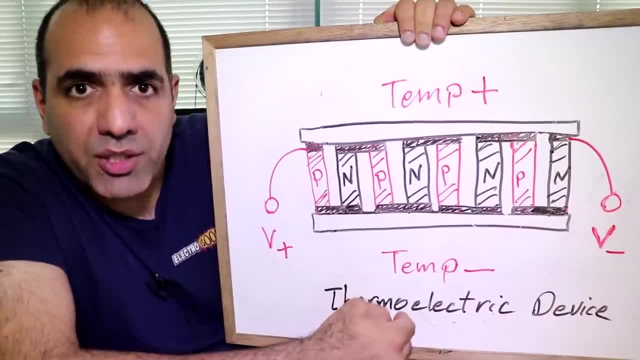 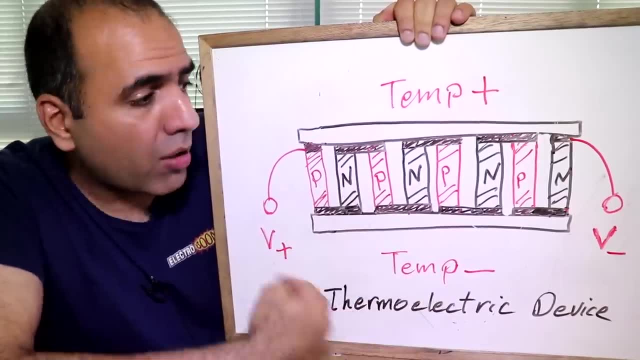 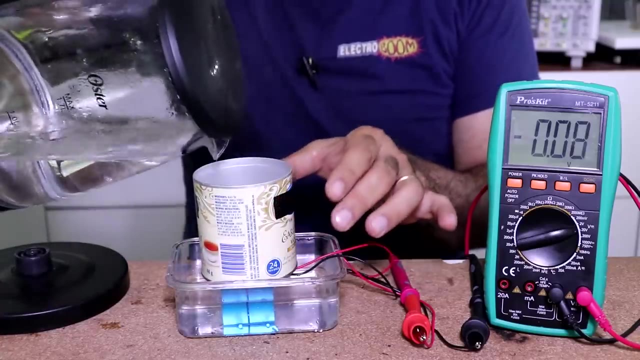 them creates a temperature difference. Also, if you place a temperature difference between the two surfaces, you create a much higher voltage because of so many junctions in series. Flipping the temperature also flips the voltage. Let's give it a try. I have a box of tea with metal bottom and if I pour boiling water, 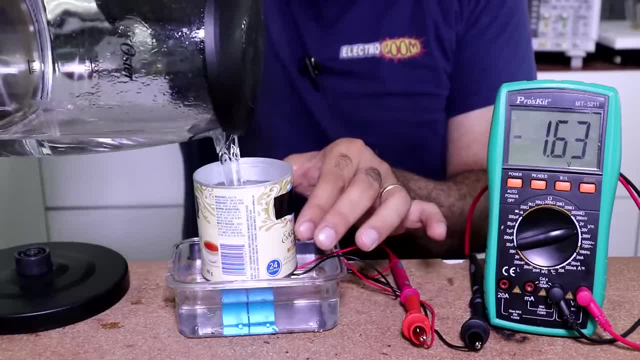 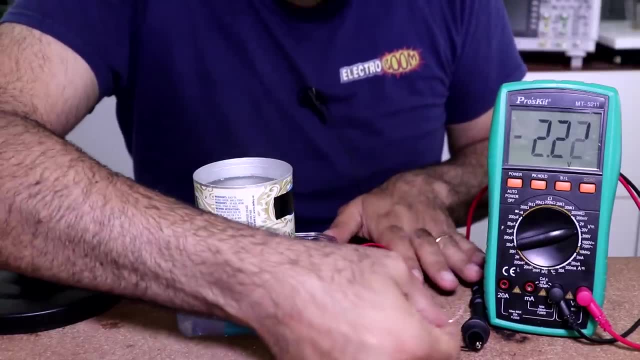 in it. I have a box of tea with metal bottom and if I pour boiling water in it it creates a voltage at the output of the device around two volts, so I can use this to power something Here. I have a 10 ohm resistor and if I connect it to the output right now I'm drawing. 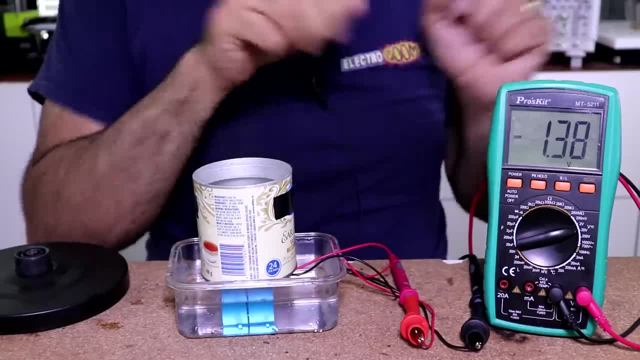 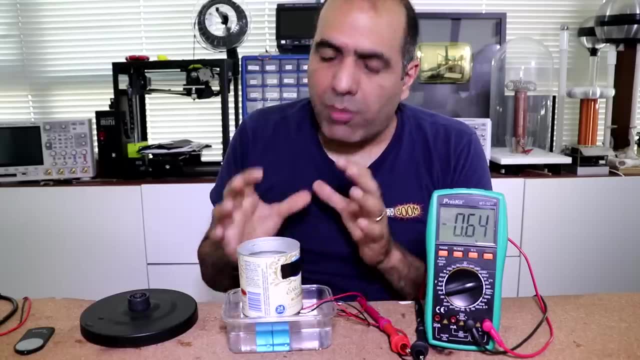 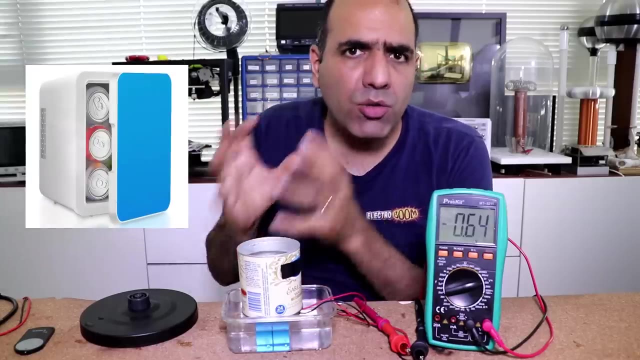 like 160 milliamps from it. Of course the voltage drops as the hot water cools down and the heat heats up and temperature difference gets smaller. In general, thermoelectric devices are pretty inefficient to create either cool or voltage. Their main application is in those small cooler. 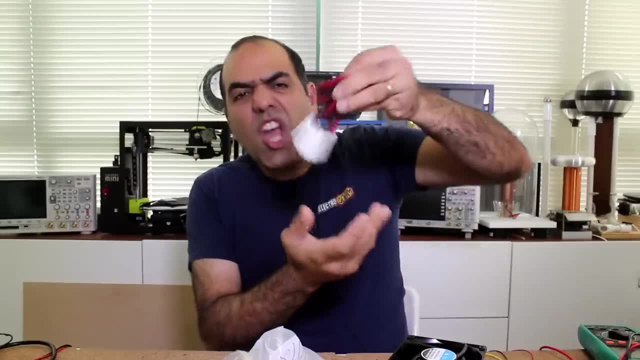 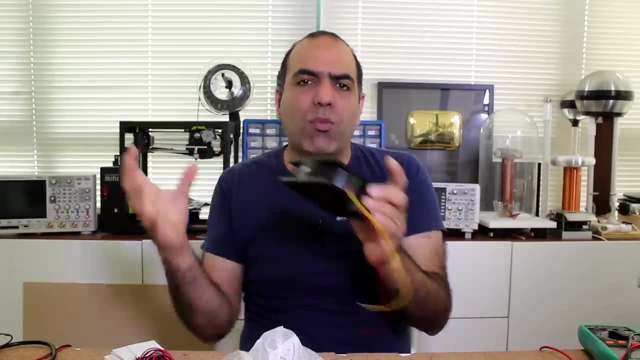 or fridges, because they are light and small. Now I want to put nine of these modules together to create a cooling surface. slash a generator if possible, and so I bought a big fan to blow on the heat sinks and a bunch of screws and a wood board. Let's put them together. 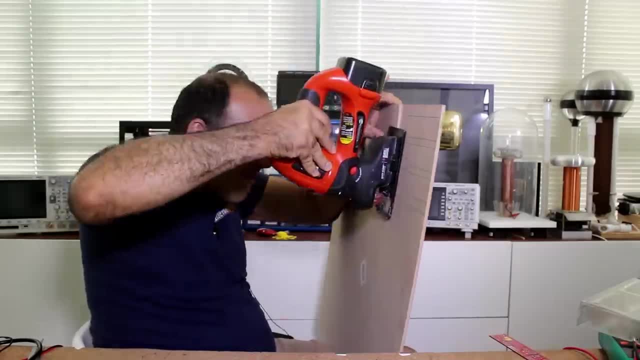 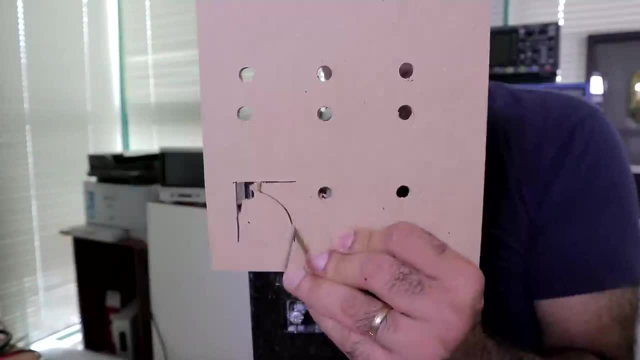 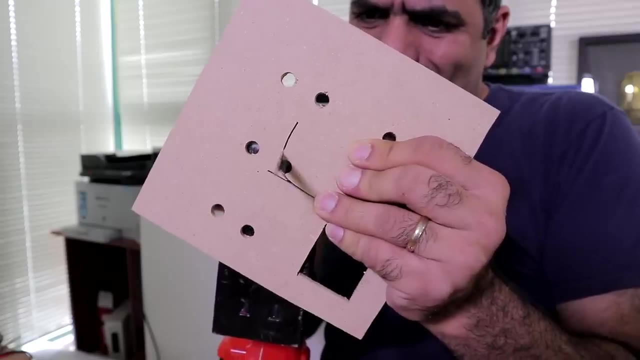 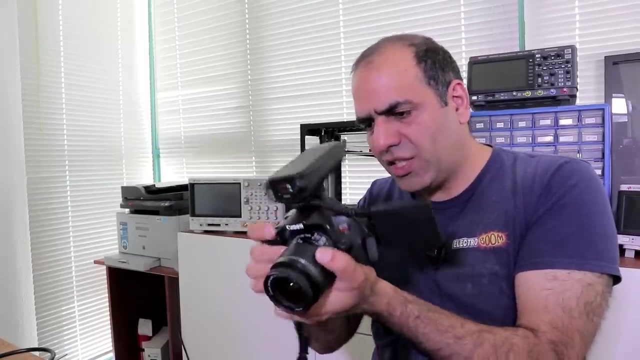 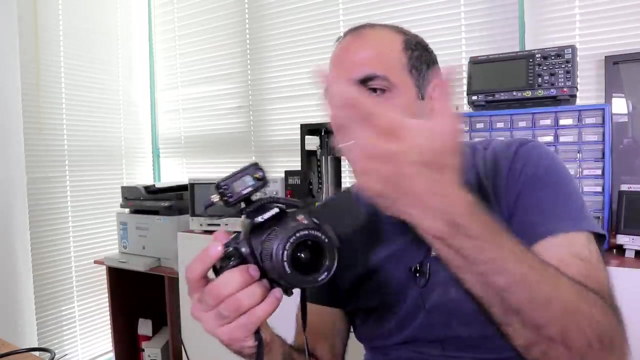 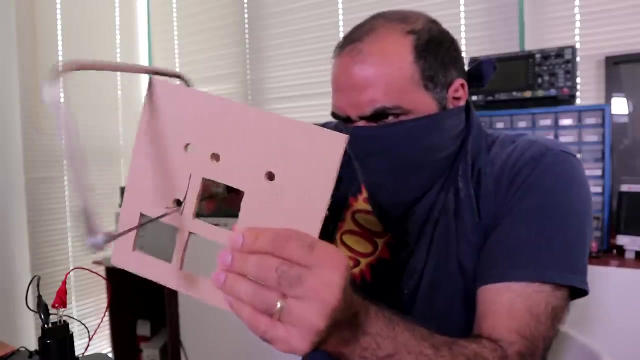 The hell. My camera of six years just blew up. Well, now I'm stuck with one camera and it doesn't have a microphone, So I can't really use my wireless lapel anymore. Audio quality down Here. my window of opportunity is made. Now I have to just install these heat sinks in it. 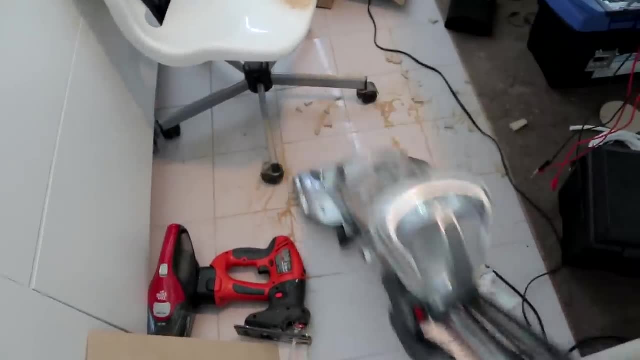 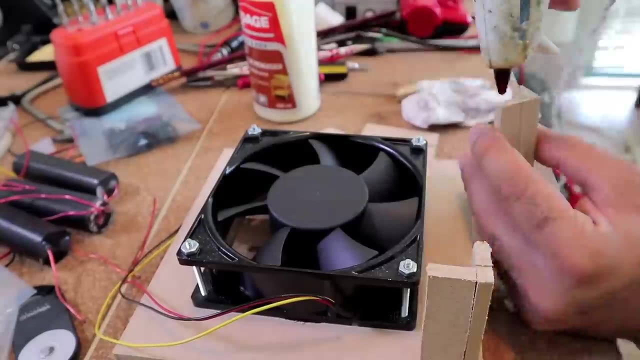 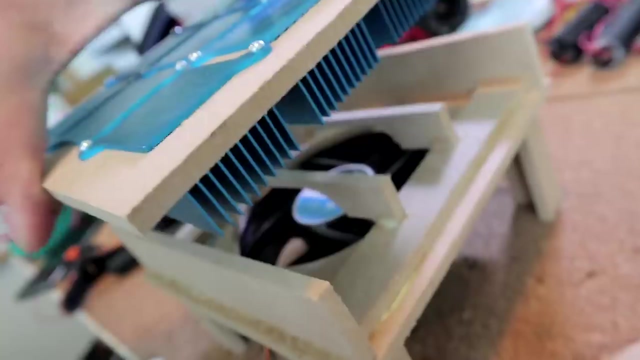 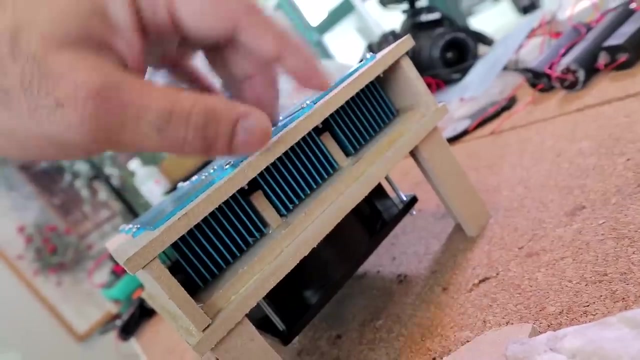 Okay, so let me show you what we've got. The fan here will blow up directly into the heat sink. I raised the heat sinks up a little bit so that the air has a chance to get over to all the fins of the heat sink, and I put those pieces of wood in the bigger channels to block them a little bit. 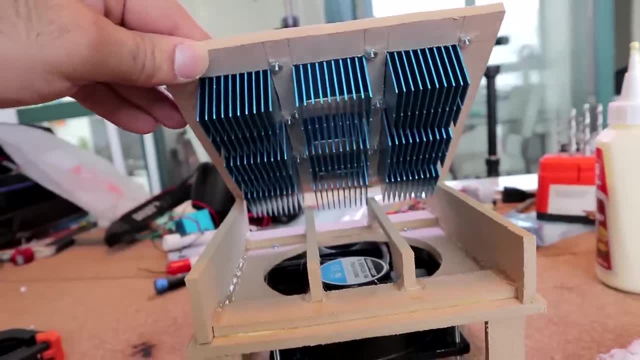 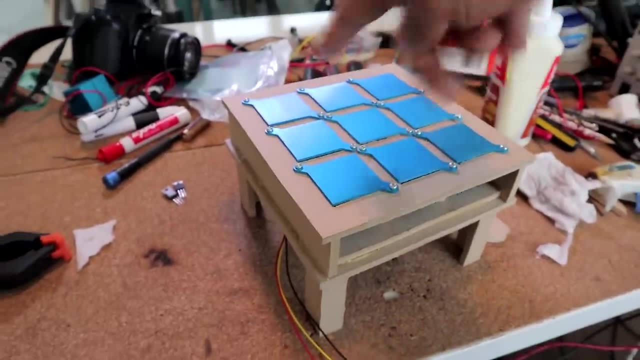 to make sure that the air gets to all the fins And the heat sinks are all in parallel, so the air escapes from front and back vents. I noticed something interesting. It seems like, because the fan is turning this way, maximum airflow is coming out this way and out that way, and there is very little airflow. 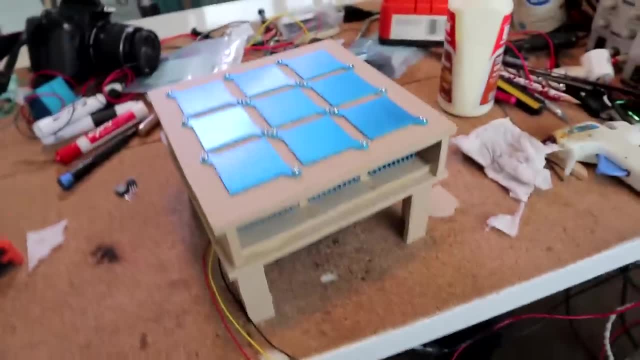 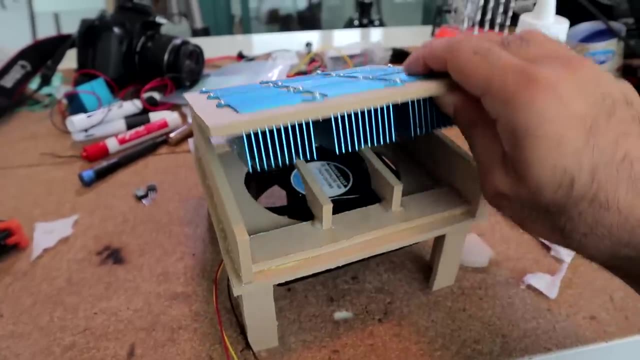 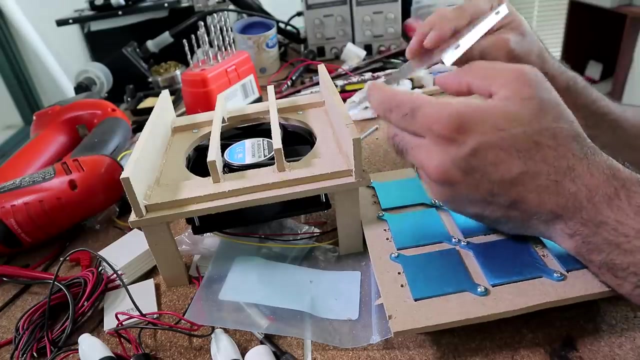 in these areas so that might affect the temperature performance of the heat sinks. So I guess the air is not just coming straight up, it's twisting, and I guess that's where the knowledge of fluid dynamics would have helped Air flow better using a cd cover. Let's hope it works. 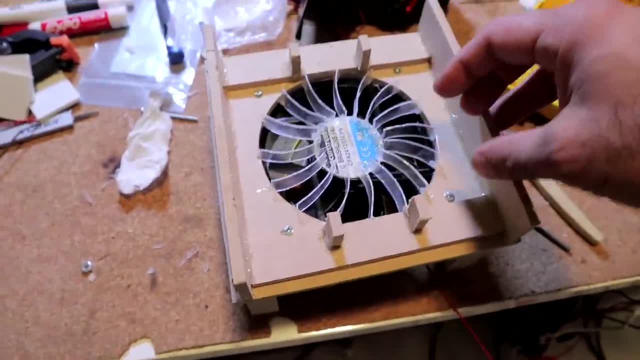 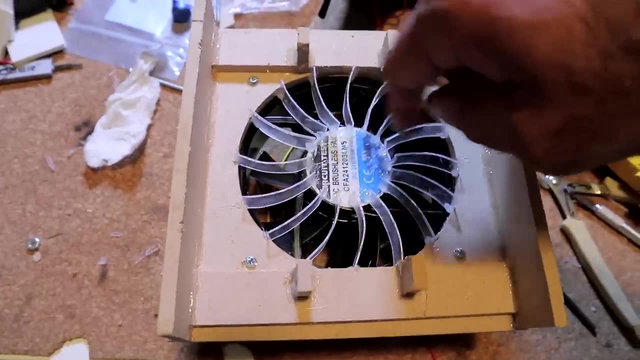 So here's what I've made for the fan, and I think I've seen it on some other fans before. Basically, my fan. when it blows, the air spins up like this. But now, with these fins, the air, instead of twisting, it will hit these walls and comes straight up. But now I've made them curved, so what? 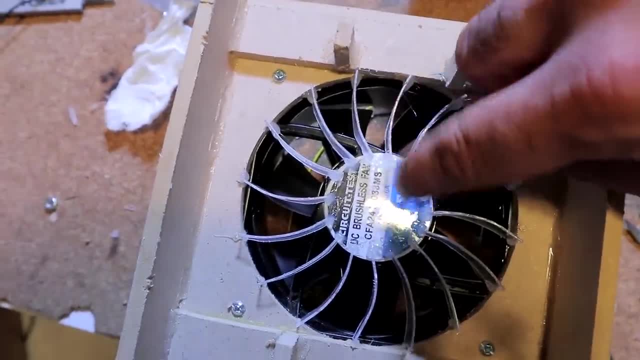 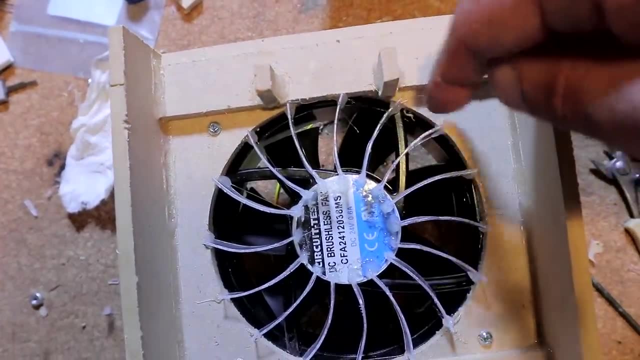 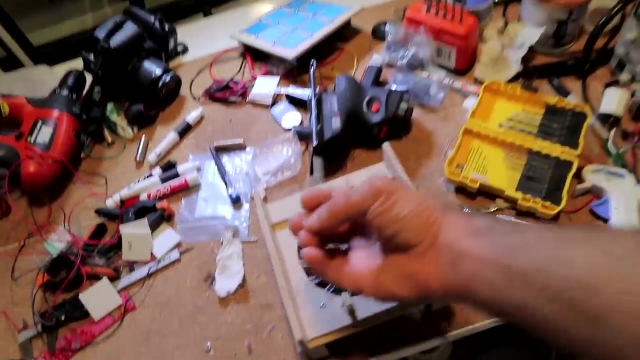 happens is that when the air hits here, it slips inside. so all these fins push the air inside, where there is almost no airflow. And when the air hits on the outside curve of the fins, it is pushed out this way so it spreads further out. So instead of one twisting column of air, hopefully it's more. 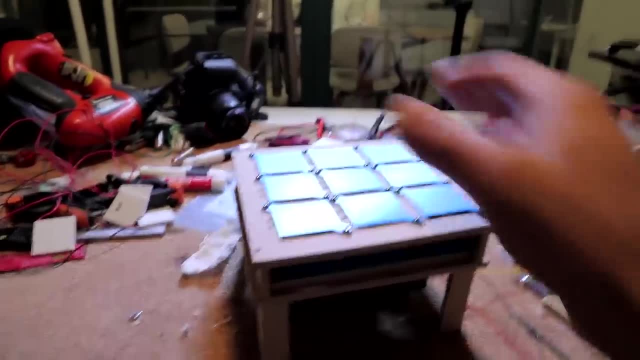 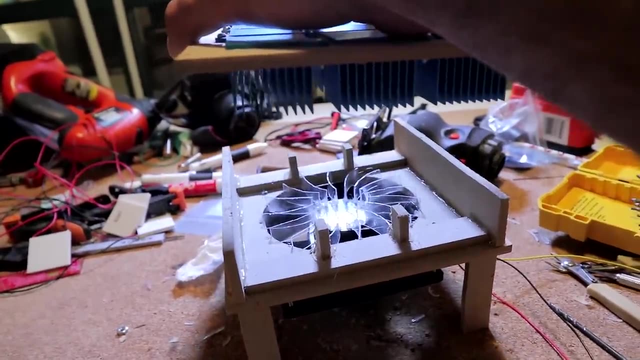 spread out and even. Okay, let's see if it helps. It doesn't really help that I placed the fan too close to the fins. You know, if there was a greater spacing between them, the air would be much more even and would cover more of the fins. Well, you know, I'm an electrical engineer. I'm not really. 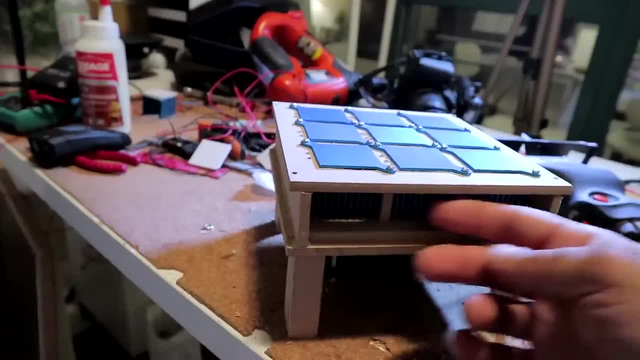 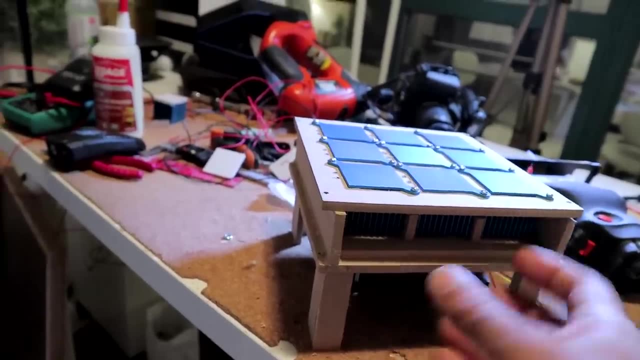 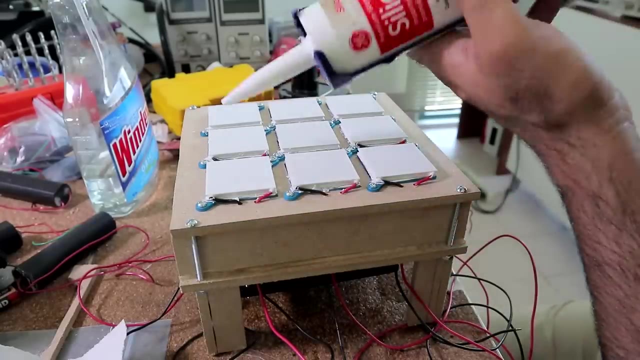 qualified to do this kind of mechanical stuff. Hey, look at this, These two. the airflow feels almost the same. This one feels a little bit less, but it's much more even now. Okay, now that everything is in place, I'm gonna cover between them with silicone, not only to keep. 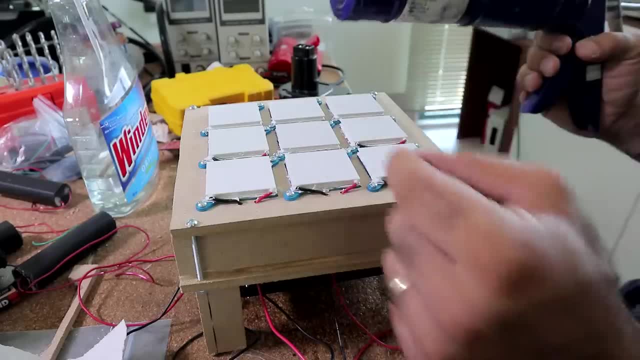 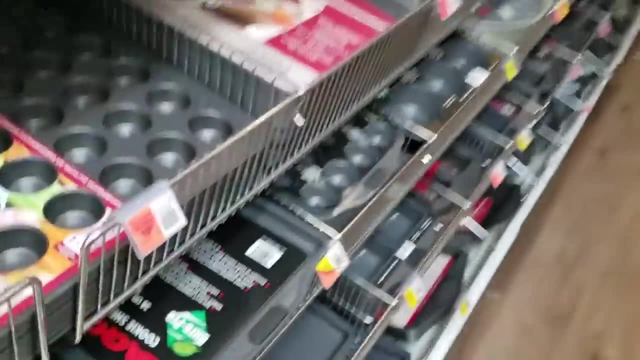 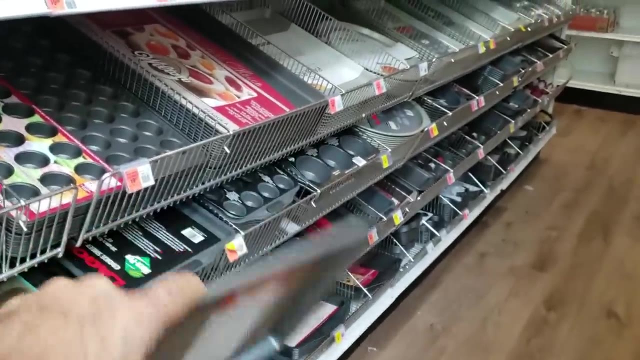 these devices in place, but also to further isolate the hot and cold surface, Or at least that's my thought. Okay, I need a small pan. I don't want to have to cut a piece of sheet metal. I want it nice and straight, like this, but small. I want something square and small. Don't seem they have it. 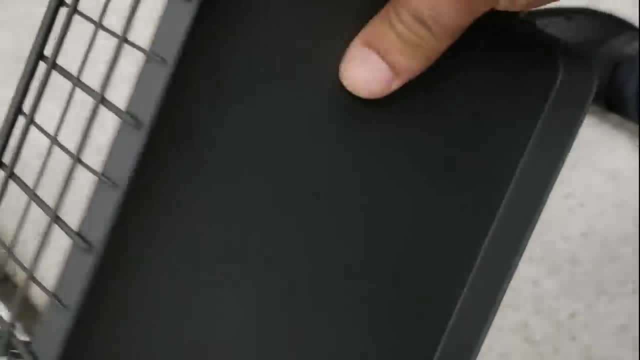 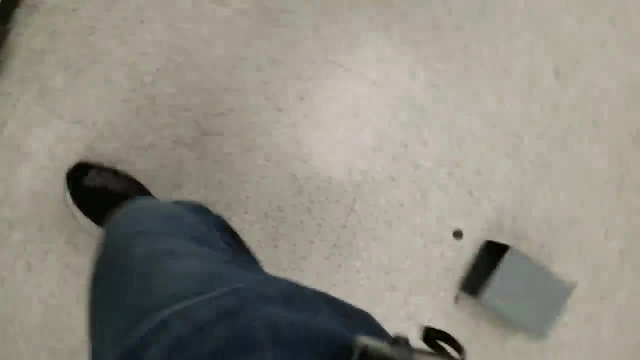 This looks good, but it's part of a napkin holder. Maybe I should just buy the whole thing and cut this out of it. Oh, these metal doors are perfect. If I can find one without the handle, Fine, I'll just buy one of these and cut it. 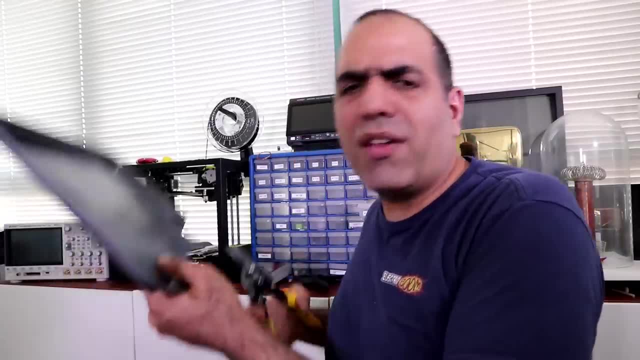 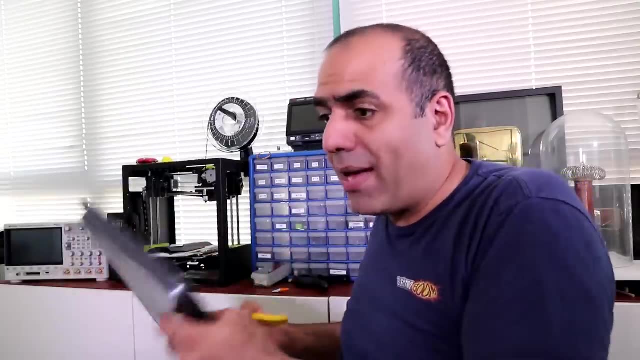 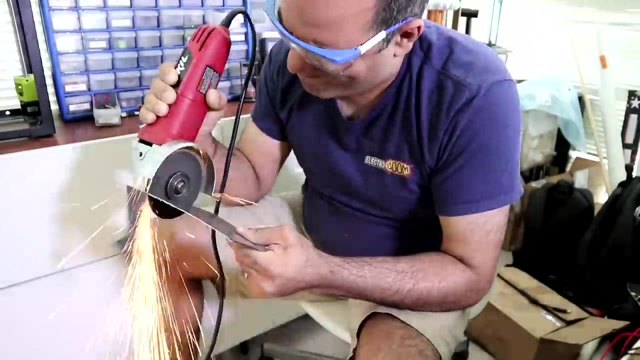 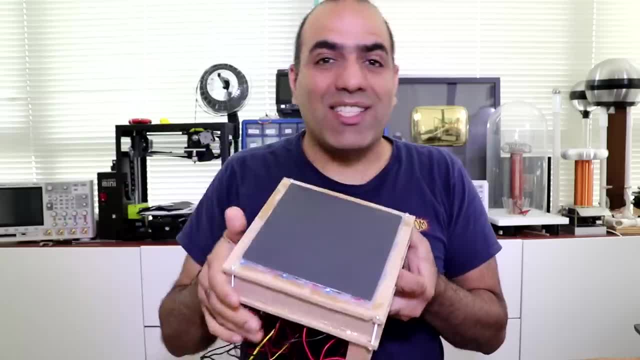 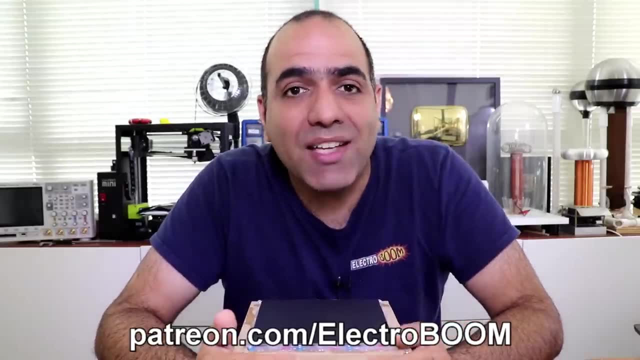 Help spread the heat evenly to all the devices, And so it's done. Just took a week or two And, thanks to my Patreon support, I got a new and improved camera. So to thank them, I'll buy them four 3D printers. Thanks for keeping my videos afloat. Now to use it as a generator. 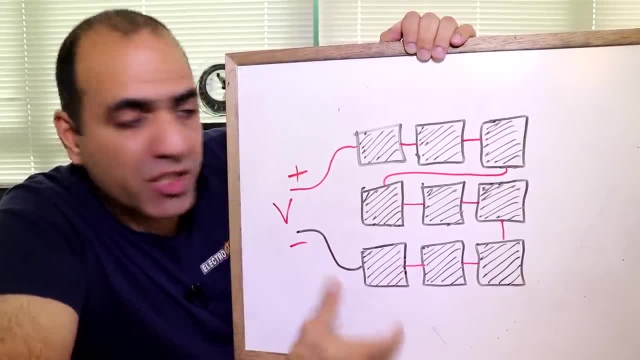 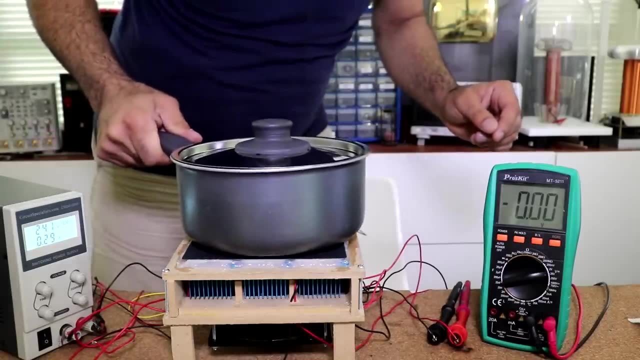 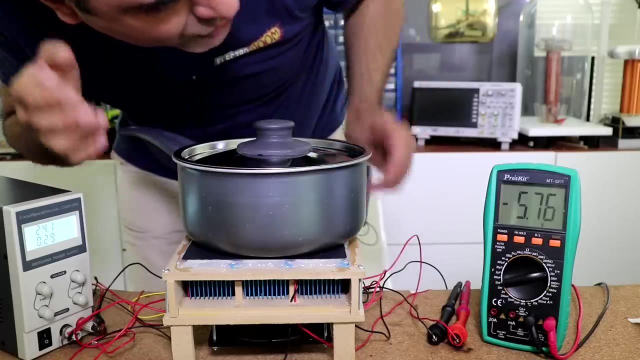 I put all the modules in series, hoping that the sum of voltages is usable. So here I'm boiling some water and with my 24 volt fan running, I put my water on top of it and that's it. I guess my heat sink in water was creating a larger difference. 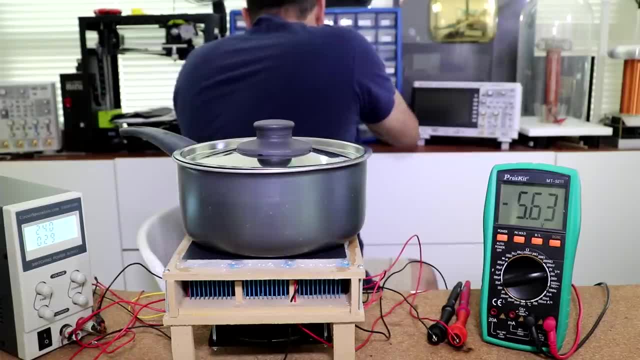 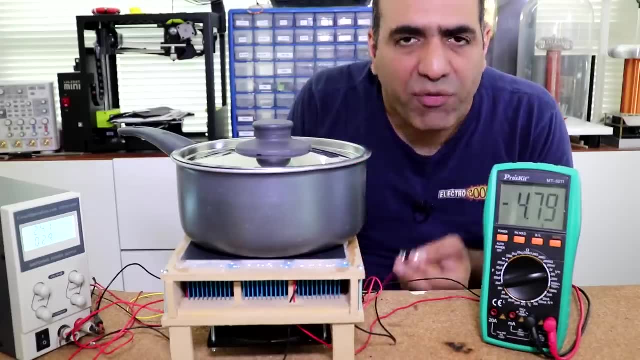 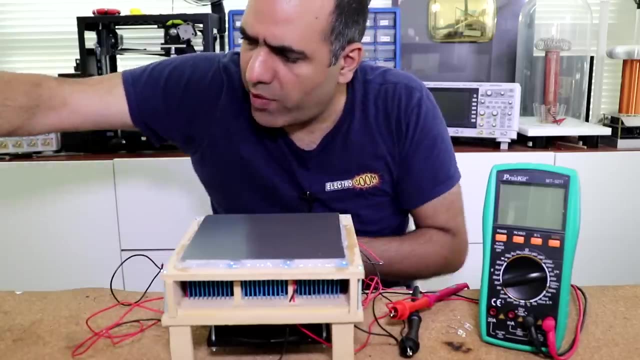 What is this good for? It's a joke. I guess I can turn on two white LEDs in series. Oh look, one of them is red. So a 24 volt fan, a pot of boiling water and hours of work to turn two LEDs on. I think somewhere it said: if the module is good for cooling, it's not good for power. 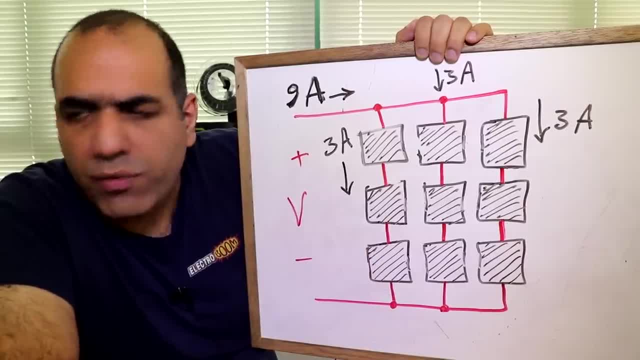 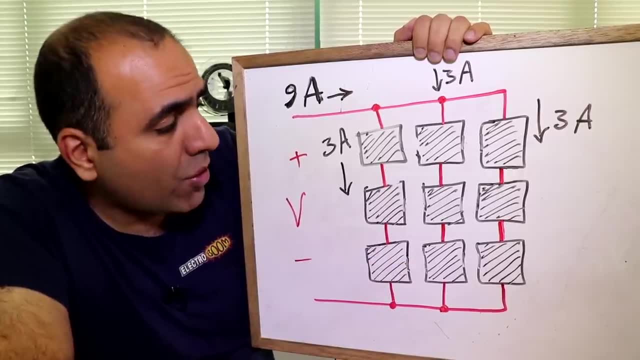 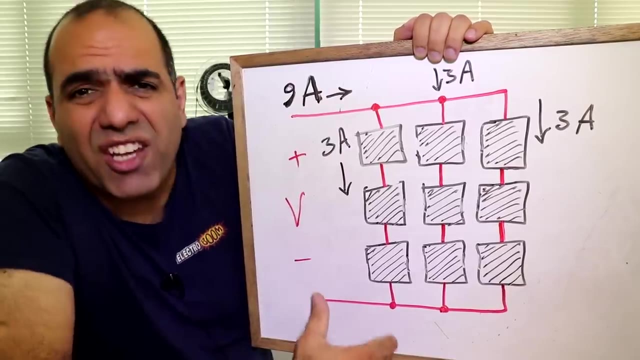 generation. So it better cool. Now to make it a cooler. unfortunately my power supply can do 10 amps maximum, while every module can take 5 amps max at 12 volts. So I put every three modules in series and put the branches in parallel so that I can at least do 3 amps per module. Not ideal, but hey. 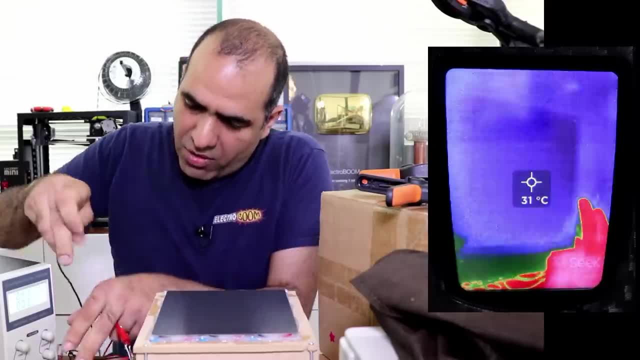 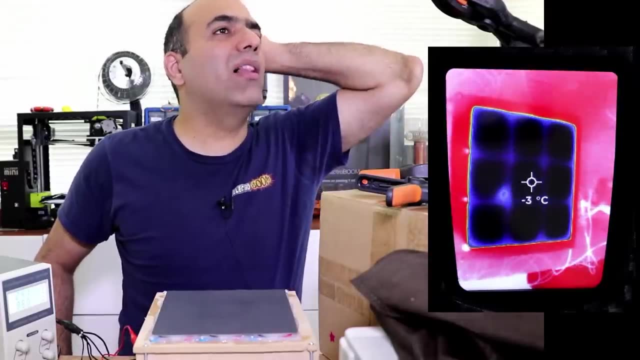 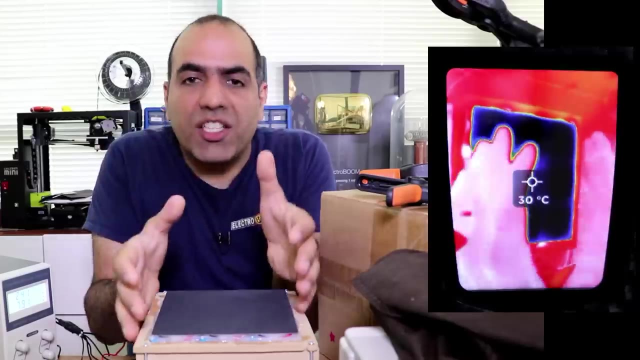 I'll run the unit and the fan at 24 volts, So 8 volts per module. Look at this. it's cooling quite well. Well, now that it's almost settled, it's running 8 amps at 24 volts, So around 190 watts. I'm sure if I contain this, it will get even cooler.